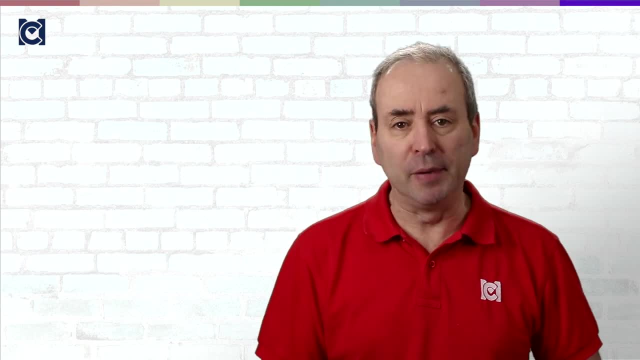 the rates for different advertising slots on their media or the procedures for bidding against competing companies to secure specific slots. With some media companies, it is usual to negotiate the first and second slots of the advertising media. The advertising media companies will then negotiate the final price for the specific slot that you want. This will depend on the type of 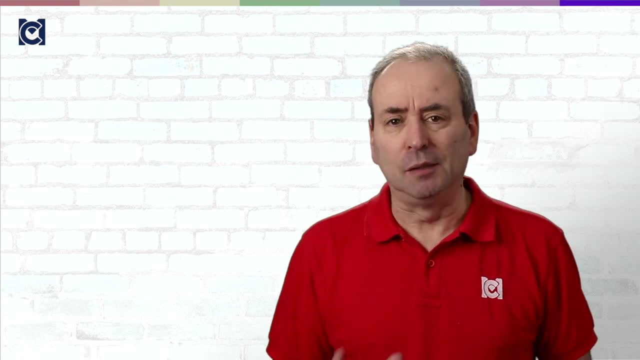 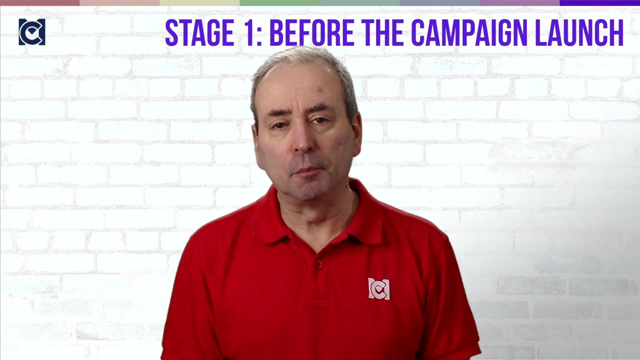 campaign, but negotiation can get you a lot. Sometimes it's as simple as an improvement in the price that you're paying. Other times it can be an enhancement in the slot that you're offered, or sometimes free or discounted additional slots, And the media buying process has three stages. 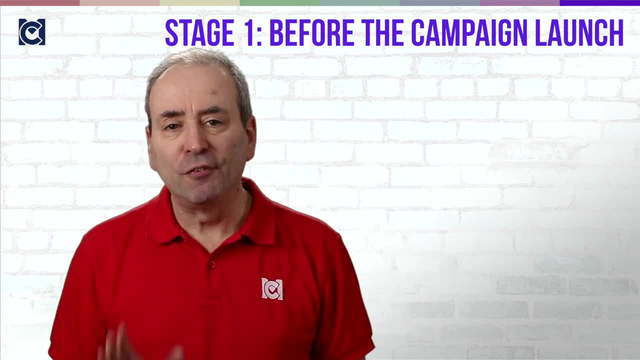 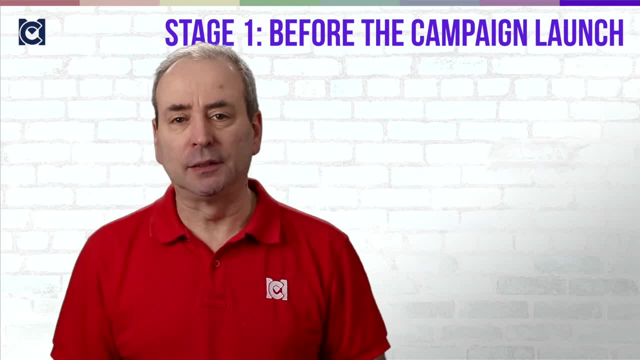 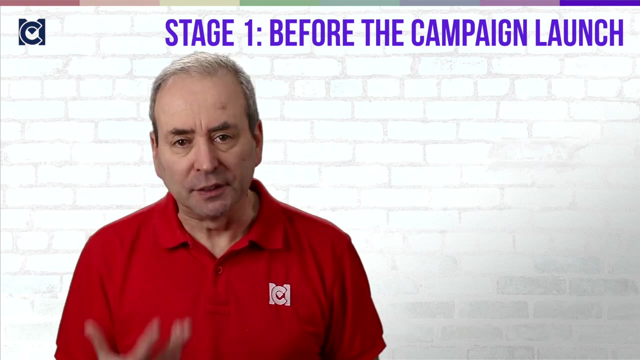 You'll also research which audience is your competitor's target and what media they use to reach them. This means you can select the right type of media channel and the specific outlets within that channel. For example, you might choose television and then you'll choose which TV channels best match your audience demograph. From this you can start to 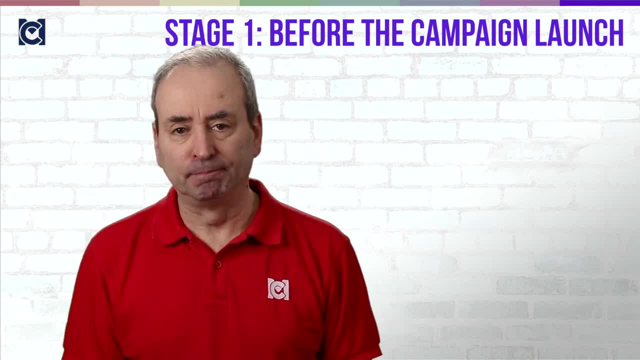 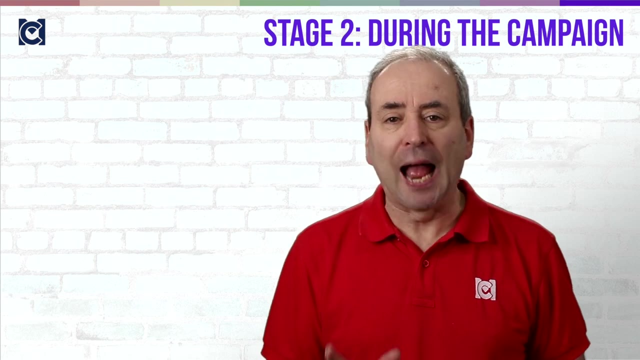 make estimates and eventually allocate a budget. And finally, in the pre-campaign launch phase, you'll buy your media placing and document the specifications in a contract. During the campaign, you will need to constantly monitor and audit the delivery of advertising against the specifications in that contract. During the campaign, you will need to constantly monitor and audit the delivery of advertising against the specifications in that contract. 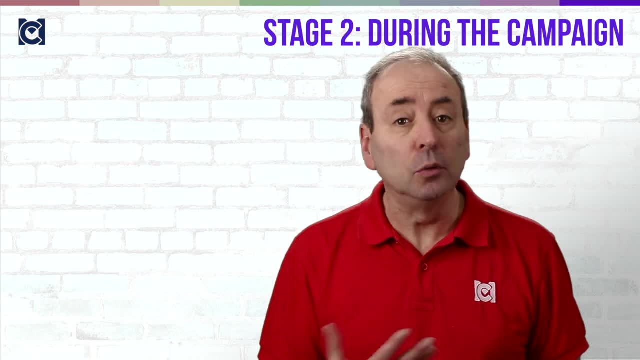 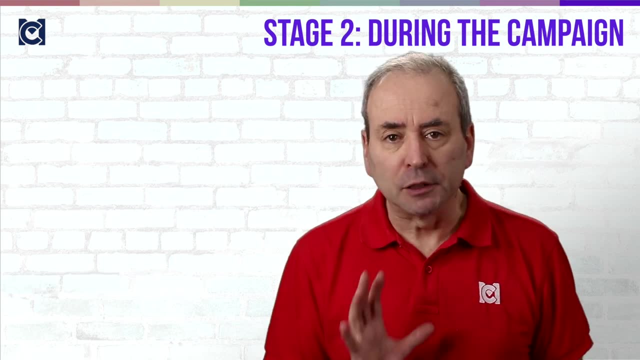 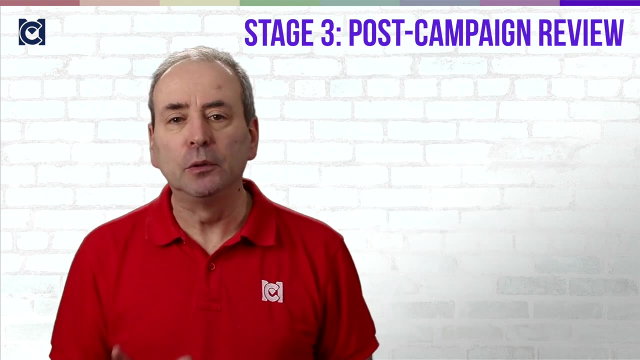 It's also worth reviewing responses from target customers and also from competitors. What are people doing, What are people saying And, of course, in response to that, you may need to revise your plan accordingly. After your campaign, you will need a post campaign review. Collect all of the campaign data.